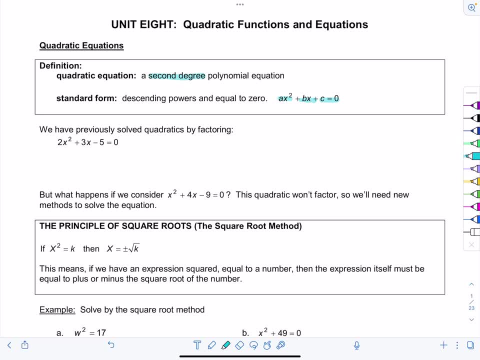 Now, we have solved quadratic equations before. Don't worry, you're not imagining things. We just solved exclusively quadratic equations that factored, So something like 2x squared plus 3x minus 5 equals zero. We would solve that square equation for the term with x squared plus 3x minus 5 equals zero. 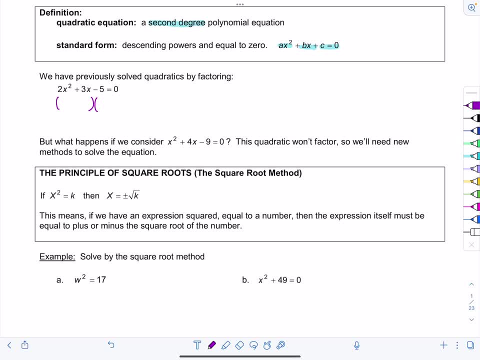 that by factoring. And let's see, do we still remember how to factor? I hope so. 2x squared, that's going to be 2x, and x 5 is 5 and 1.. Let's try this way out. That's going to be good. 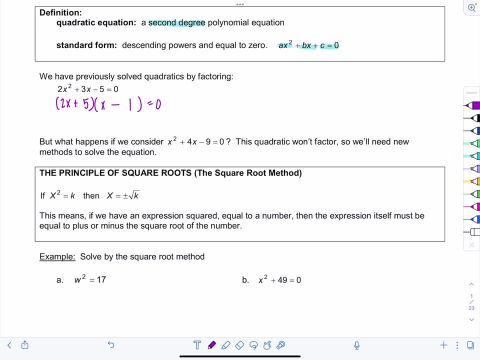 Plus 5 minus 1.. And then, remember from here, we used the zero product property, which- let us set each of the factors separately- equal to zero. So 2x plus 5 equals zero, or x minus 1 equals zero, And then from there we could get our solutions: x equals negative, 5 halves. 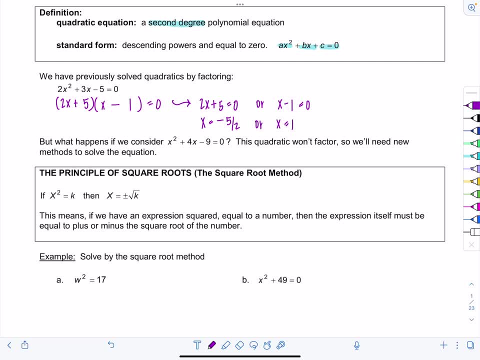 or x equals 1.. But what happens if we consider the following quadratic equation, Something like: x squared plus 4x minus 9 equals zero. This quadratic equation will not factor. So what does that mean for us? We don't just give up. No, no, no. 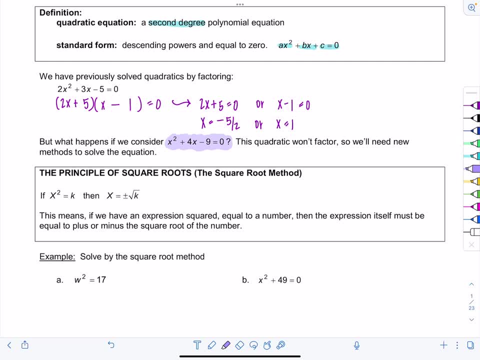 We just need to factor. We need a new method to solve the equation. So first we're going to start off with the principle of square roots, which is the square root method, And it states the following: If x, squared, equals k, then x equals plus or minus the square root of k. 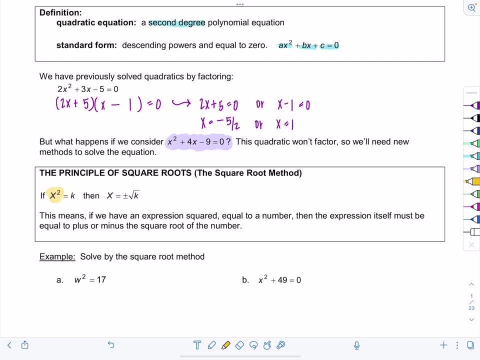 And you might notice, I've got this giant capital X squared here, because it doesn't necessarily refer to just the variable x. If you just have some sort of expression that's squared equal to a number, then you're going to get the square root of x squared. 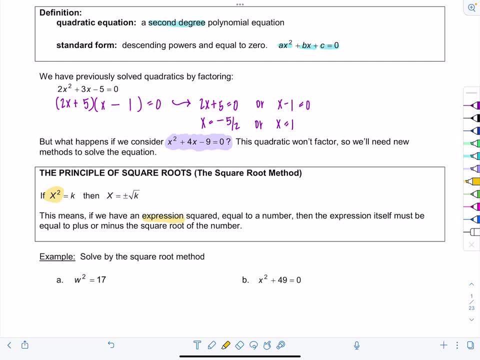 Then that means the expression itself must be equal to plus or minus the square root of the number. So let's work through some examples so you can see exactly how to use this square root method, And we're going to learn different methods for solving quadratic equations At the end of learning. 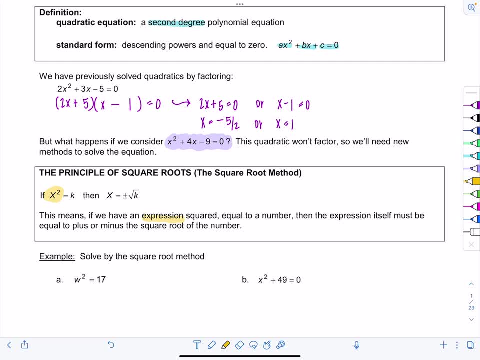 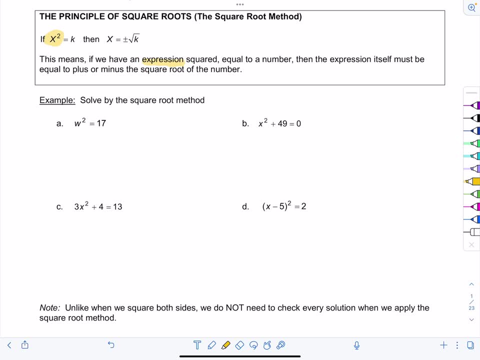 them all. we'll talk about when is the best time to use each one, But for right now, let's just focus on this square root method. So we've got w, squared equals 17.. You always want to make sure that the squared expression is always equal to the square root of the number, So we're going to 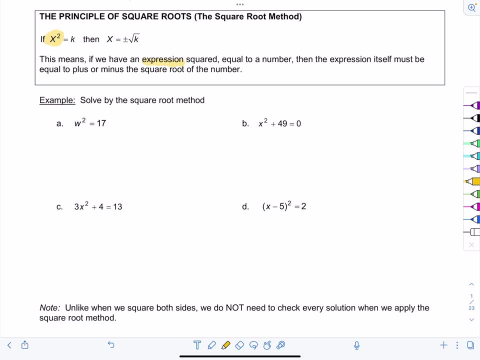 go ahead and take the square root of both sides and always put the plus or minus in front of the side where the constant is, And we're pretty much done right. That means w equals plus or minus the square root of 17.. And square root of 17 doesn't simplify any further, so that's it. 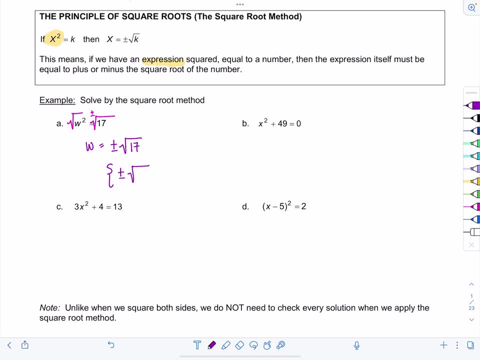 If you want to put it in a solution set, go for it. I like to. All right, next one: x squared plus 49 equals 0. We can already tell that's not going to factor. A sum of squares is prime. So what do we do? Let's isolate the squared quantity, meaning I want. 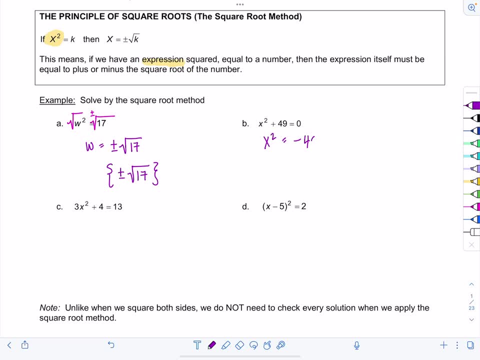 x squared all by itself constant on the other side. So now it's a negative 49.. We can go ahead. Let's take the square root of both sides and then put the plus or minus in front where the constant is Okay. square root of x squared, that's going to give us x, And this equals plus or minus. Now be: 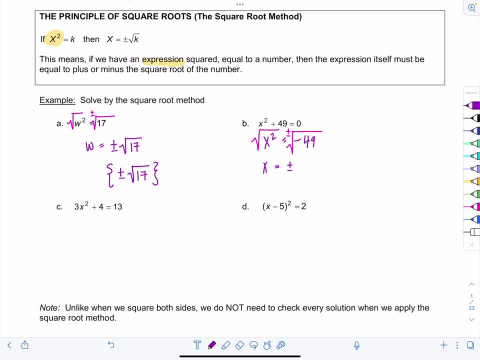 careful, since there's a negative underneath the radical, then we're going to have to attach the imaginary unit i to our answer. So square root of negative 49 is going to be 7i. All right, so those are our solutions, plus or minus 7i, Not too bad. Let's look at a couple more: 3x squared plus 4. 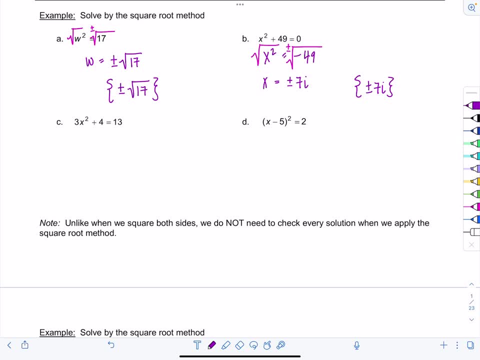 equals 7i. So we're going to have to add the imaginary unit i to our answer. So square root of x squared equals 13.. So in this case I want to isolate the squared quantity as much as possible. Let's start off by subtracting 4.. So we've got 3x squared is equal to 9. And then divide by 3,. 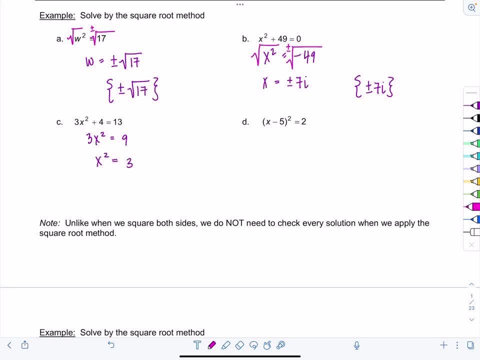 which means x squared is equal to 3.. Now it's square root time. So take the square root of both sides plus or minus over here And we're left with x equals plus or minus square root of 3.. Okay Yeah, I love my solution sets. Last one example D. We have x minus 5, quantity squared. 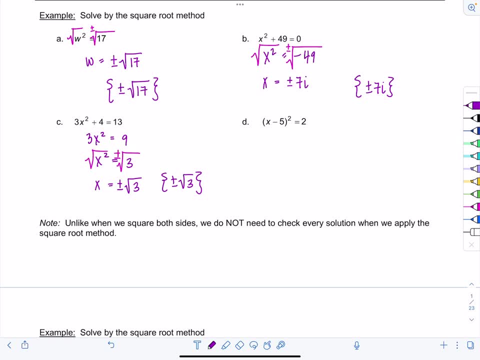 equals 2.. Notice, I have a squared expression on the left side. It's not just a variable all by itself, But it's all good. I can go ahead and take the square root of both sides right now. Don't do something wild like multiply this all out, because then you won't be able to use the. 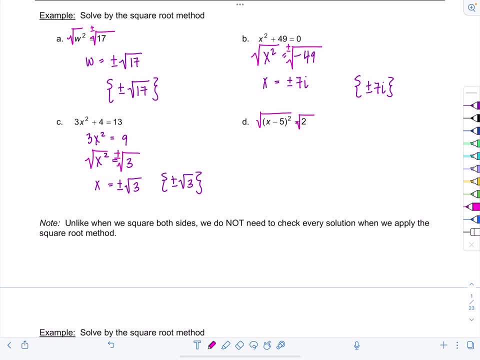 square root method. We actually love it the way it's written right now: Square root, plus or minus. Now I have x minus 5 equals plus or minus the square root of 2.. Good To get the variable by itself. you just got to add 5 to both sides, So now we have x equals 5. 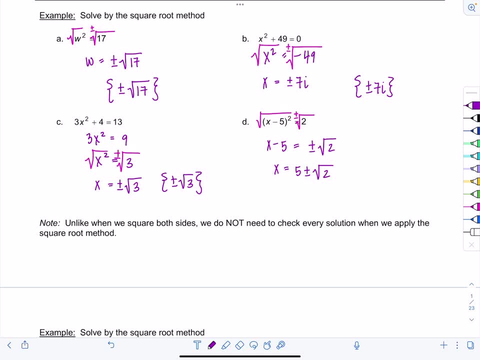 plus or minus square root of 2.. And that's your final answer. Okay, You wouldn't put plus or minus square root of 2 plus 5.. That's just not the way it's done. Okay, And in the previous video that we worked on, we solved radical equations And when we squared 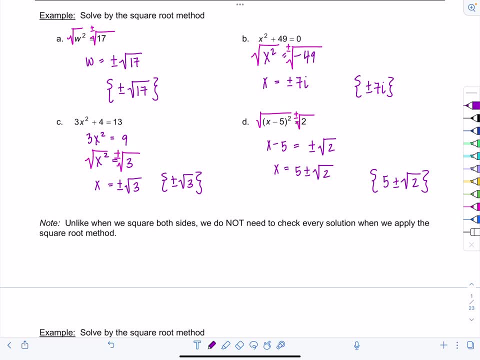 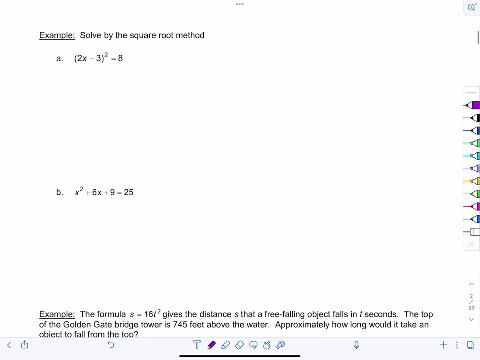 both sides, we had to check every solution. That's not the case here. When we take the square root, no need to check every solution. Okay, A couple more spicy ones Again. solving with the square root method, We've got 2x minus 3. quantity squared equals 8.. Why don't you guys? 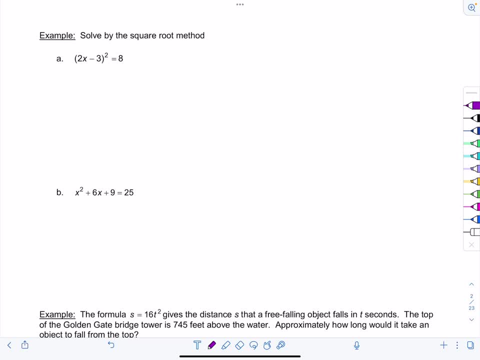 pause the video. Give this one a try on your own. I have faith in you. You can do it, Okay. So let's see what we've got. Take the square root of both sides, Put a plus or minus over here where the constant is, And now we have 2x minus, 3 equals plus, or. 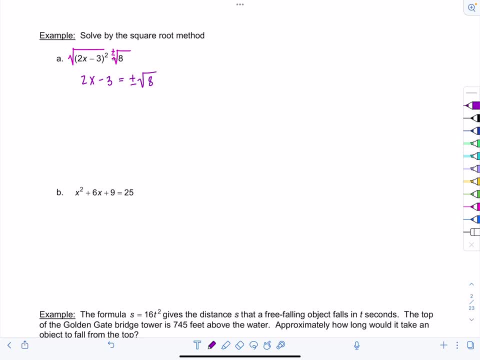 minus radical 8.. But wait a minute. Radical 8 simplifies right, It's 4 times 3.. So we've got 2x minus 3 equals plus or minus 2 rad 2.. Very, very good. Add 3 to both sides. We're trying to get that x all by itself. So we have 3 plus, or. 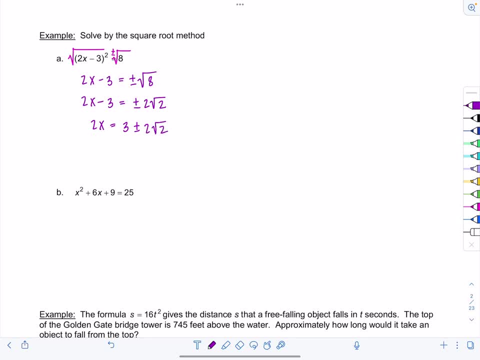 minus 2 rad 2.. And then, last step: let's divide everything by 2.. So x equals 3 plus or minus 2 rad 2 over 2.. Good, Now, don't be tempted to do something illegal, like maybe cancel these 2s out. 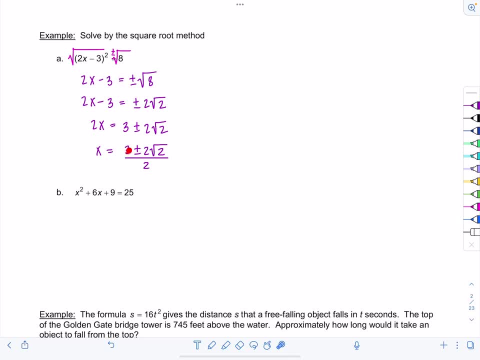 because you can't cancel. You can only cancel a 2 out from the 3 over here. Okay, So it just wouldn't be fair. It would actually be illegal. The math police would come after you. So you can only cancel out if, say: 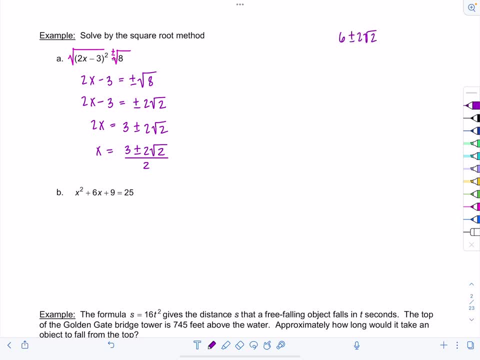 for example, you have something like 6 plus or minus 2 rad 2 over 2.. Then if you factor that 2 out from everybody in the numerator, then you can go ahead and cancel out the 2 in a legal fashion. 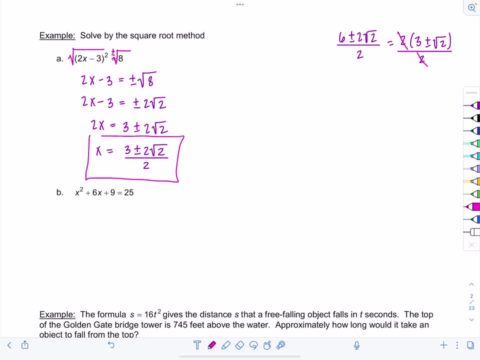 But the way it's written right now, please refrain. Okay. So let's just go ahead and put the answer in a nice little solution set before you're tempted to do something wild. So 3 plus or minus 2, rad 2, all over 2.. Good, 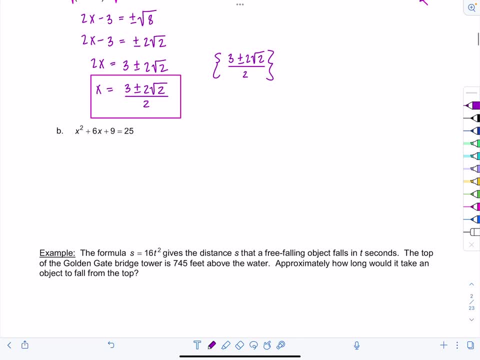 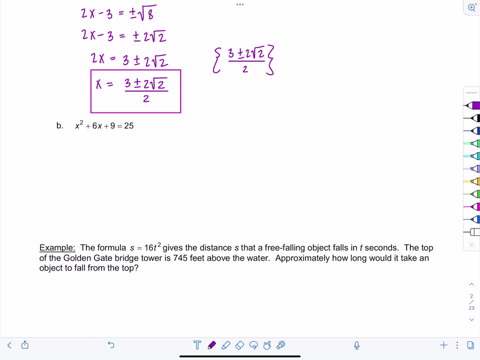 All right. Next, we've got example B. Again, we're solving by the square root method And we have x squared plus 6x plus 9 equals 25.. And you might think, wait a minute, How are we going to use the square root method? 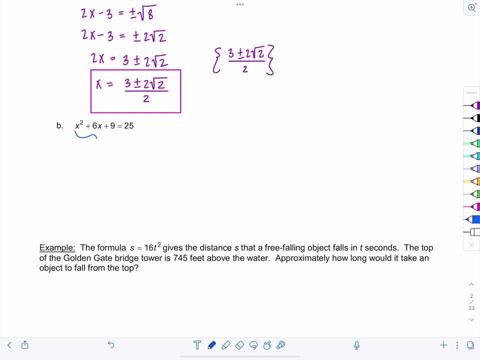 But observe: x squared plus 6x plus 9 is a perfect square trinomial. What does that mean? It factors into x plus 3 times x plus 3, also known as x plus 3 squared. Oh, lucky for us. Okay, So then? 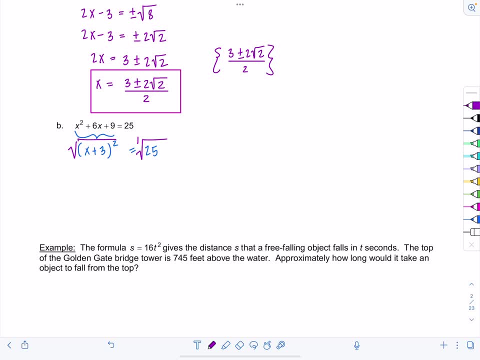 now I can just go ahead and take the square root of both sides. This is working out nicely. And then we've got x plus 3 equals plus or minus. square root of 25 is just 5.. Okay, Getting x by itself. Now we have x equals negative, 3 plus or minus 5.. 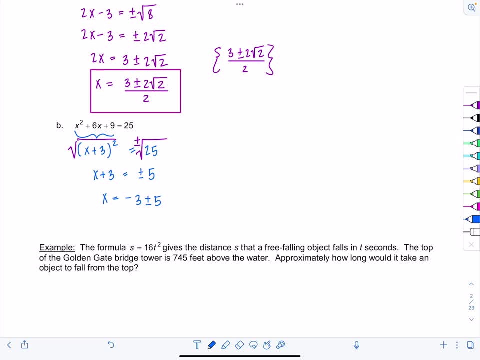 Oh, but we don't stop there, because 5 isn't underneath a radical or anything, So that means we can simplify further. It's going to be negative 3 plus 5,, which is 2,, or negative 3 minus 5,, which is negative 8.. So those are our two solutions. 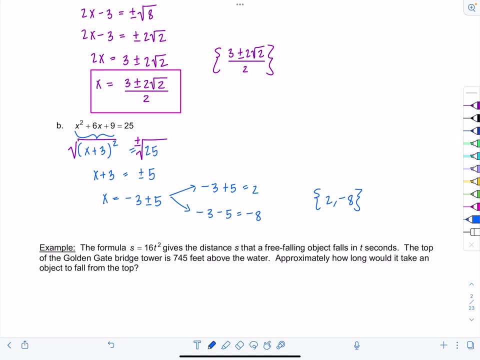 Notice. they were rational, which means we could have solved this equation just by factoring. But you know, a lot of success in math hinges on just being obedient and following directions. So that's what we're here for, people. Okay, How are we doing Good? All right, Let's look at a 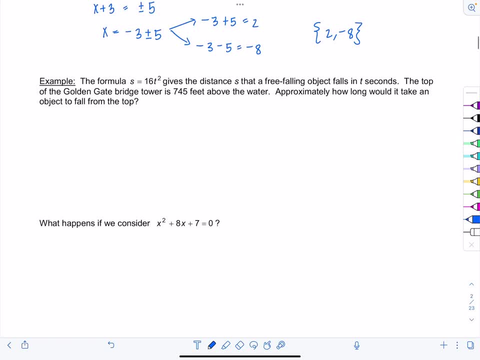 little word problem, Just a cute one. The formula s equals 16t squared gives the distance s that a free-falling object falls in t seconds. If you've had some physics, this is no surprise to you. The top of the Golden Gate Bridge tower. 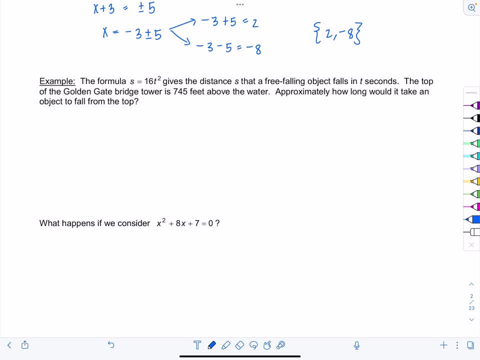 is 745 feet above the water, Approximately, how long would it take an object to fall from the top? And let's just round to one decimal place, Okay, Okay, So we're going to use the formula s equals 16t squared, And they want to know how long it's. 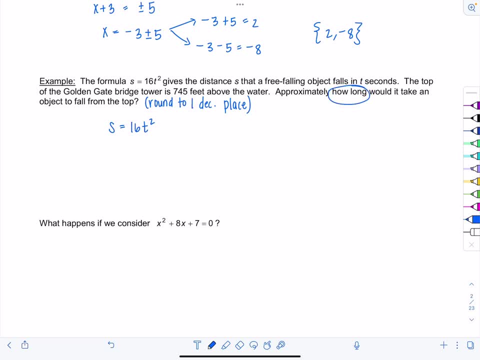 going to take. So we're going to solve for t for an object to fall from the top. So that means the distance that it would fall would be the full 745 feet. So 745 equals 16t squared. Let's solve by. 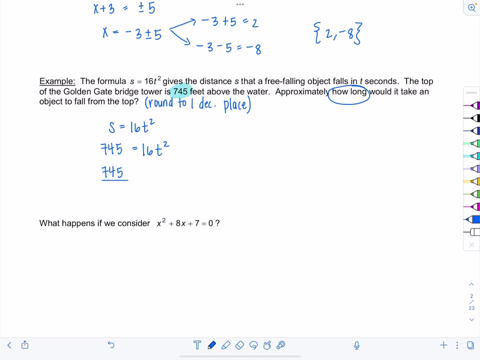 the square root method. So 745 over 16 equals t squared. Let's take the square to both sides. I'm going to put plus or minus, But as of yet- when this video is recorded in 2022, we can't travel backwards in time, So we're only going to use the positive radical for our 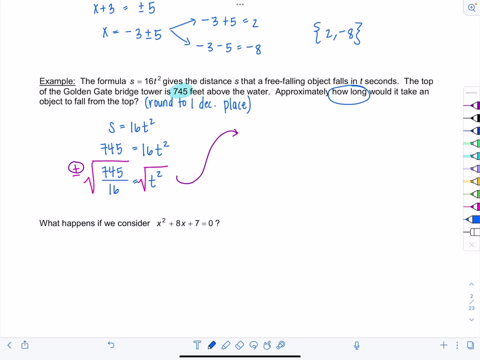 solution: Okay, So that means t equals. and let's split that- radical 745 over radical 16.. So that means t equals rad 745 over 4.. I'm not going to fuss with trying to simplify the radical, I'm just going to punch it in the 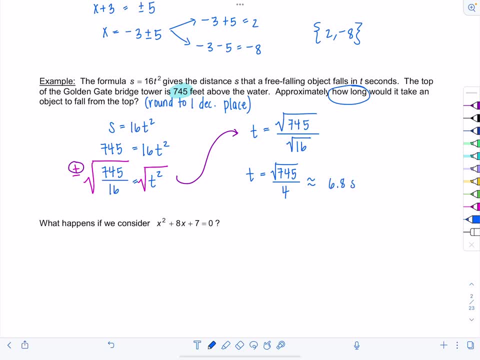 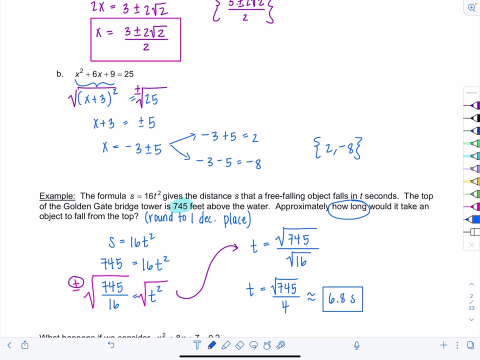 calculator and we get approximately 6.8 seconds. That's quick, huh Man. Okay, now back to the idea of using the square root method. Remember how we were super lucky with that last example- x squared plus 6x plus 9, because we already had a perfect square trinomial. 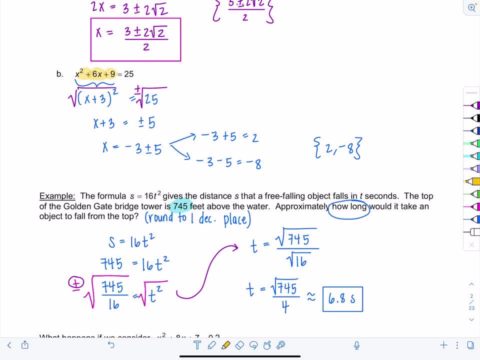 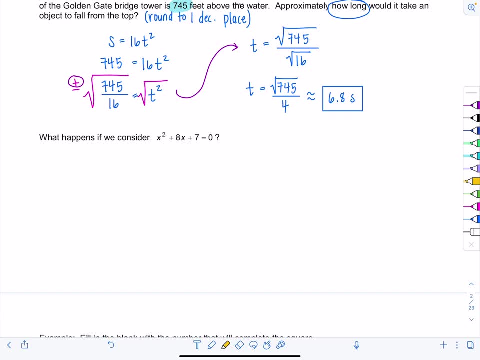 handed to us. Life will not always be so sweet, my friends. So what if we had something instead that was x squared plus 8x plus 7 equals 0, and you still had to solve by the square root method? I know it factors, I know it's so tempting, but let's be. 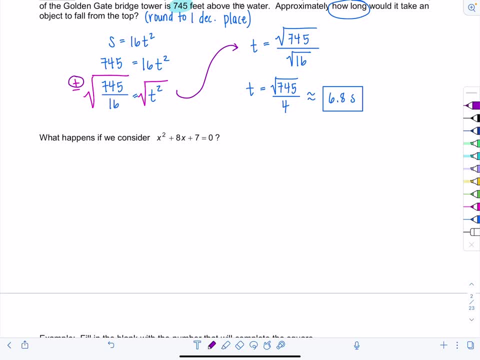 obedient little math students. Okay, well, let's see here. I don't like the 7. It's not letting me factor into a perfect square trinomial, so let's get rid of it. you know, Ew, go away 7.. 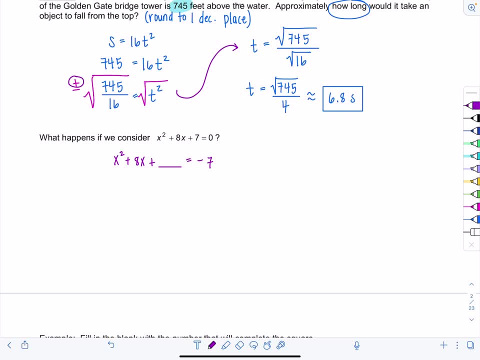 What do you wish was here instead of a 7?? How would you make a perfect square trinomial? Think about it. Think about it. Wouldn't a 16 do the trick? Hmm, I'm going to put a 16 on both sides, right, If I add it to the left. I got to. 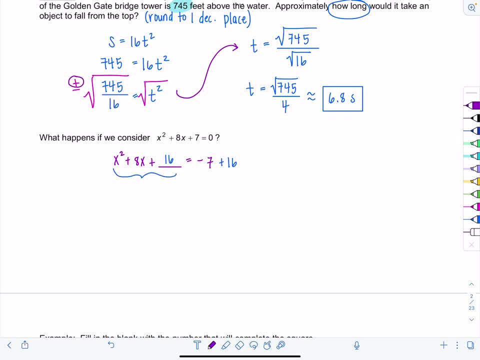 add it to the right, because now I could factor the left-hand side as x plus 4 squared, Ah, and then negative 7 plus 16, that's 9.. Oh, perfect, Now we can go ahead and use that square root method: put the plus or minus, and then we get: x plus 4 equals plus or minus 3.. 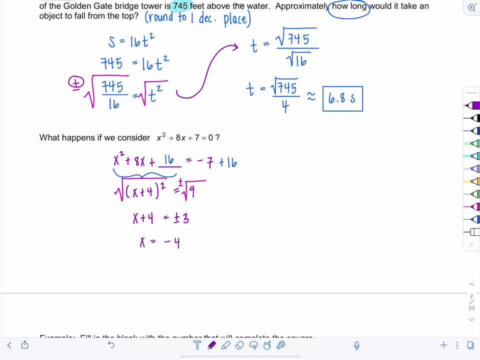 So that means x equals negative 4 plus or minus 3.. Those I can combine right: Negative 4 plus 3 is negative 1, negative 4 minus 3, negative 7. So those are our two solutions. So how exactly did I? 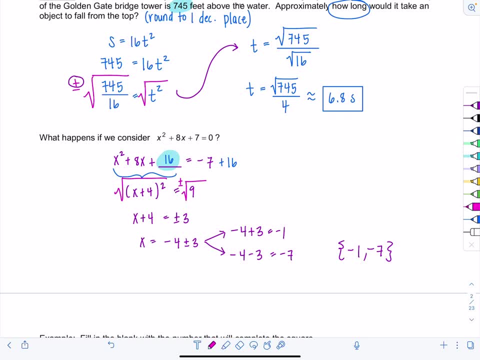 do with 16? Well, basically, I looked at this constant here in front of x the 8. And I knew, when I factored into a perfect square trinomial, it needed to be half of that, right, And so you. 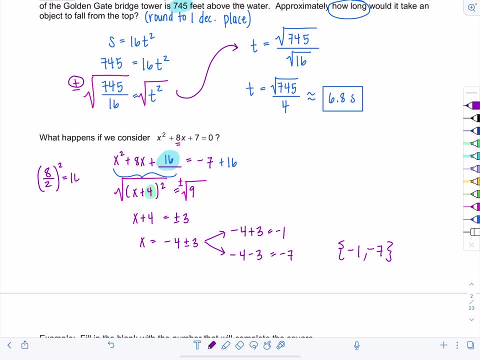 divide that number by 2 and then square it, and that's where the 16 comes from, And this process is called completing the square. So let's just practice that a couple times and then we'll go back to solving quadratic equations. 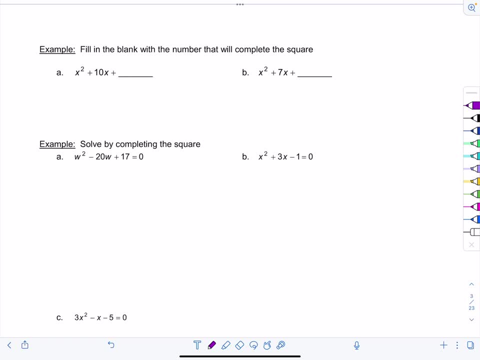 Using that method. So fill in the blank with the number that will complete the square. So you pay attention here: 10, okay, Divide that by 2,, excuse me- and then square it. So 10 divided by 2, that's 5 squared, is going to give us 25.. And then make sure you still know how. 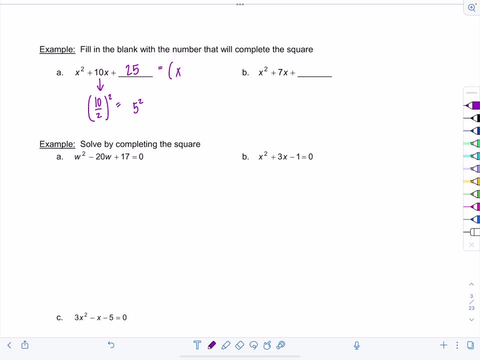 to factor after you've completed the square. So it's going to factor into x, Whatever the sign is in front of that linear term that's going to go after x, So plus, and then, in this case, 5 squared. okay, Good, Let's try another: x squared plus 7x plus blank, So again. 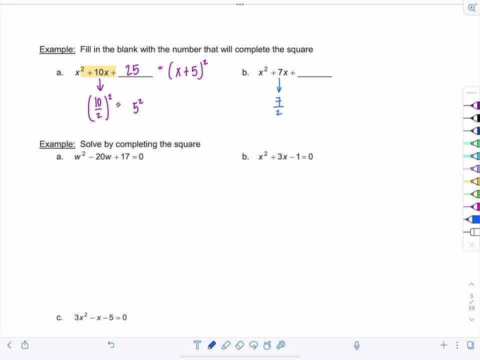 take that linear coefficient 7, divide it by 2, and then square it. So what do you get? 49, over 4.. Square the numerator, square the denominator. How would that factor x plus 7 over 2 squared? Okay, good, Fancy, fancy. So now let's go ahead. 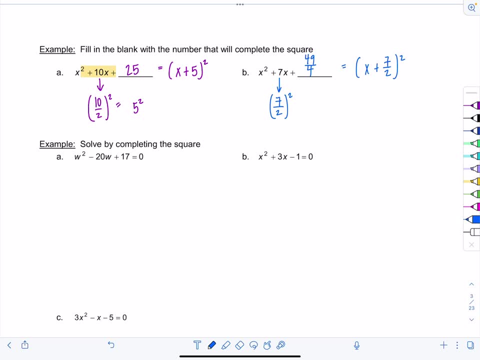 Since we can complete the square. that means we can solve any quadratic equation using that method and then applying the principle of square roots, where we can take the square root of both sides of an equation. Okay, solve by completing the square. We've got w squared minus 20w plus 17 equals 0.. 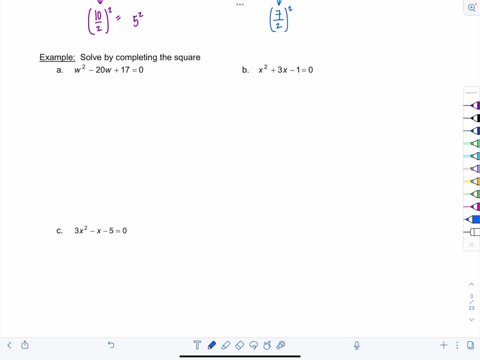 So get rid of the 17. He has no business being there on the left. So w squared minus 20w equals negative 17. And then I'm going to add something to both sides to complete the square. So let's think here: Negative 20 divided by 2, that's negative 10.. 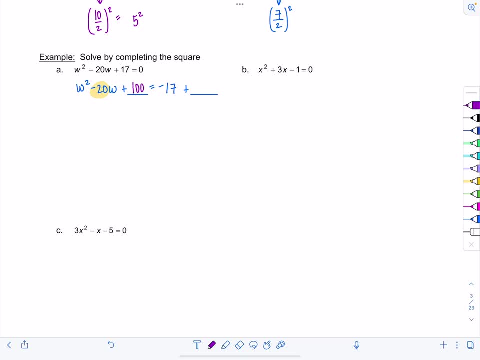 And then if I square that, I get negative 10.. So I'm going to add something to both sides. I'm going to add 100 to both sides. Good, Now let's factor. So left-hand side is going to factor into w minus 10. quantity squared equals negative 17 plus 100.. Yep, that's 83.. 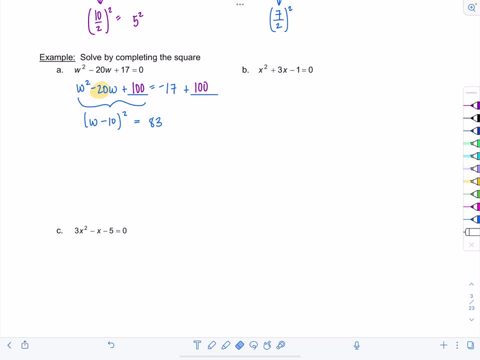 Okay, looking good. Now it's square root time, So let's take the square root of both sides. Don't forget your plus or minus, And we've got w minus 10 equals plus or minus rad 83.. Does rad 83 simplify at all? 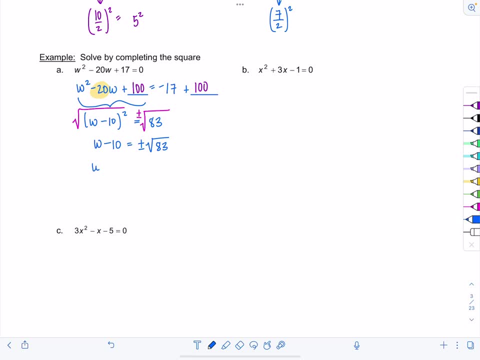 No, So then we're pretty much done. Add 10 to both sides w equals 10 plus or minus rad 83.. How was that one? Not bad, not bad, Good, Okay, example: b: x squared plus 3x minus 1 equals 0.. 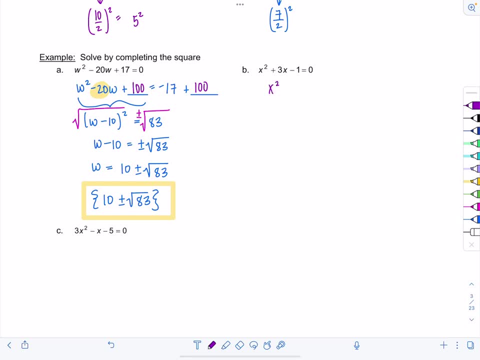 All right. So we've got here x squared plus 3x. Get that one out of there. Go over there one. Add your blank on both sides. Okay, 3 divided by 2 squared. Don't get flustered, because there's fractions. Compose yourself. 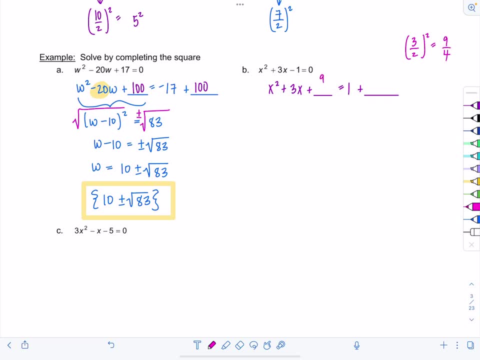 This is going to be 9 over 4.. Add that to both sides. Okay, still there, Look at you, You can do it. Okay, how is the left-hand side going to factor x plus 3 over 2, squared Good. 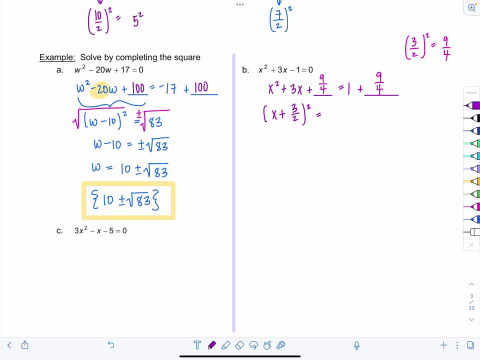 On the right-hand side, 1 plus 9 over 4.. Remember, 1 is 4 over 4.. 4 over 4 plus 9 over 4.. That's 13 over 4.. Good, Now it's square root time. How exciting, Square root, square root. 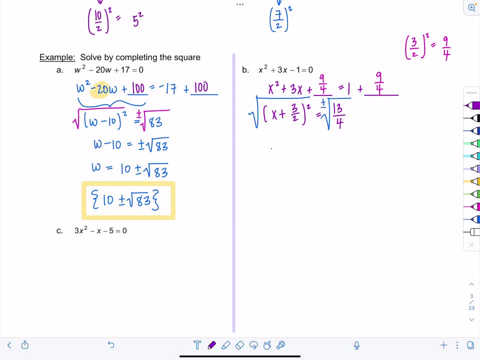 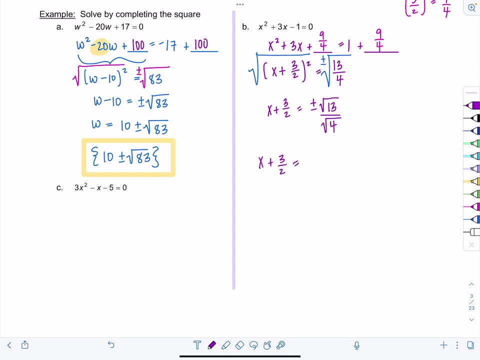 plus or minus. Now we have x plus 3 halves equals plus or minus rad 13 over. Let me split this up. Let me break up the fun Rad 4.. Okay, So that means x plus 3 halves equals plus or minus rad 13 over 2.. I'm going to subtract 3 halves. 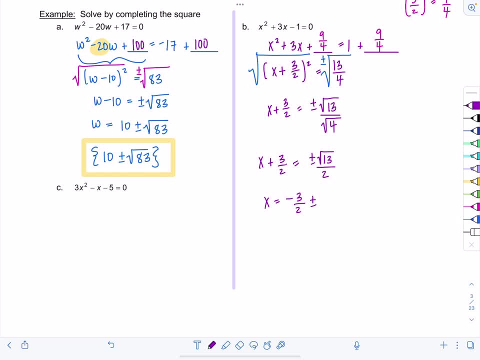 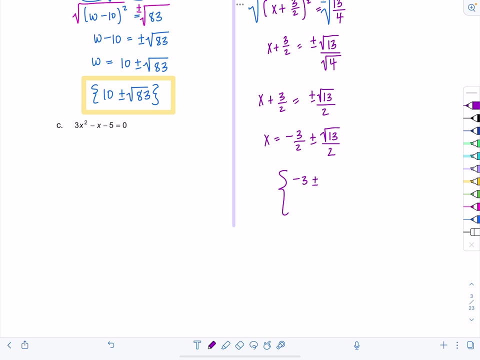 So x equals negative 3 halves plus or minus rad 13 over 2.. But notice, both those terms on the right now have a common denominator, So why don't we just put them all over 2?? So let's write our final answer as negative 3 plus or minus. 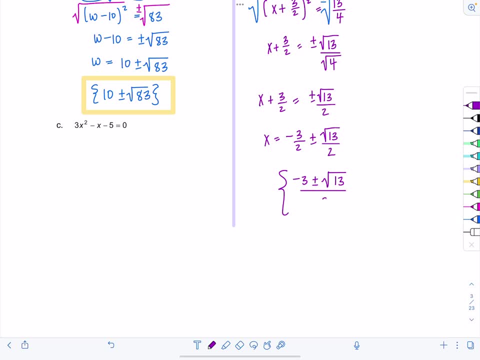 Rad 13, all over 2, like that. Oh, yes, That's the desired way to write your final answer. All right, Good, We're going to end on a high note. I've got a really spicy little one for you. 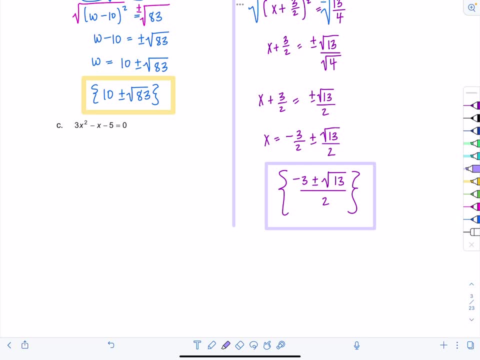 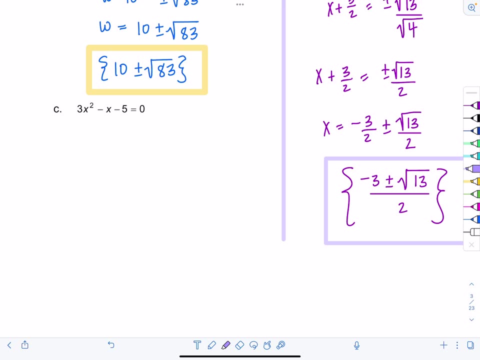 3x squared minus x minus 5 equals 0.. What is different- I mean the major thing- is the fact that there's a coefficient. So we're going to write the coefficient on x squared And we only complete the square when the coefficient on x squared is a 1.. So we've got to fix that pronto, All right. So just, we have. 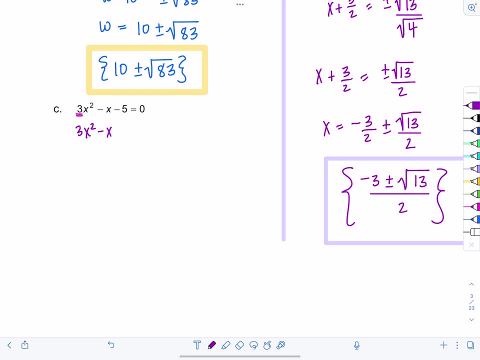 some prep work to do: 3x squared minus x, get that 5 out of there equals 5.. To make the coefficient on x squared a 1, we're going to divide everybody by 3.. Okay, So yeah, we're going to have to deal. 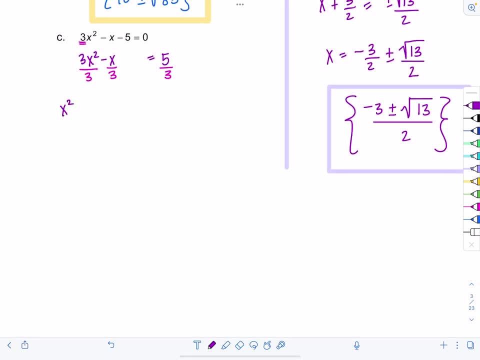 with fractions. They're just a part of life. people x squared minus 1.. So we're going to divide everybody by 3.. 1, 3 x plus something equals 5, 3.. So let's figure out what's going to go in the blank to complete the. 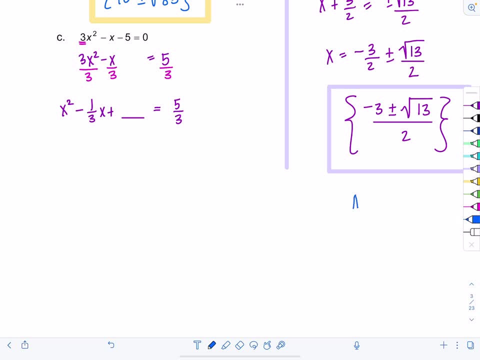 square. Let me do it off to the side here. So you take the coefficient of the linear term negative 1: 3. We're going to divide it by 2.. When you're talking about a fraction, dividing by 2 is the same as multiplying by a half. I think it's easier to think of it that way. 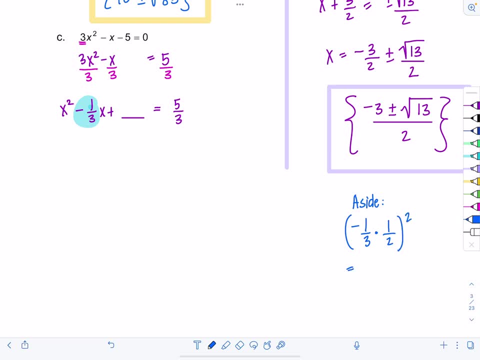 In this case. And then we square that sucker. So this is going to be negative 1, 6 squared, which becomes square. the top square the bottom: 1 over 36.. So that's what we're adding to both sides: 1 over 36.. Oh my, Okay, Now let's factor. So left-hand side is going to be x. 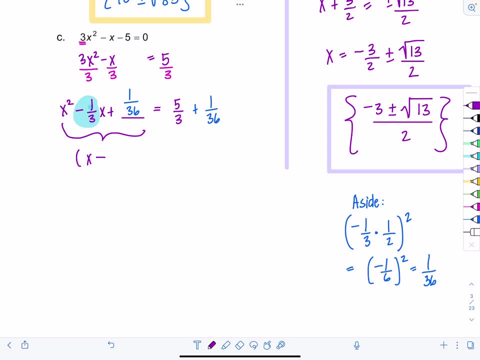 Since the 1- 3 was negative, we're going to have a minus sign. next, Always put the square root of this number, or whatever it was before you squared it, right there when factoring. So 1, 6 squared equals. Okay, Let's get a common denominator over here: 5, 3.